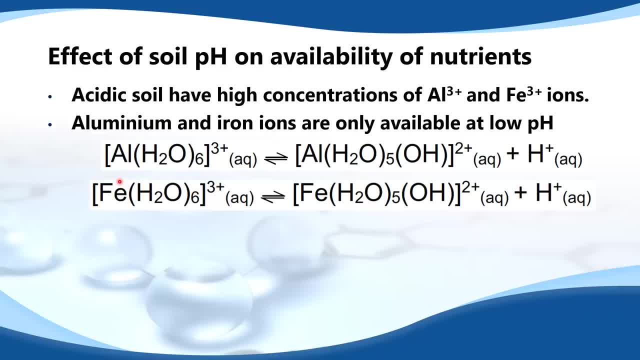 charge density of the Al3 plus and the Fe3 plus ion. they form weakly acidic solutions At high pH. the equilibrium in these two reactions here shifts to the right as the H plus ions are removed from solution by the OH negative ions in. 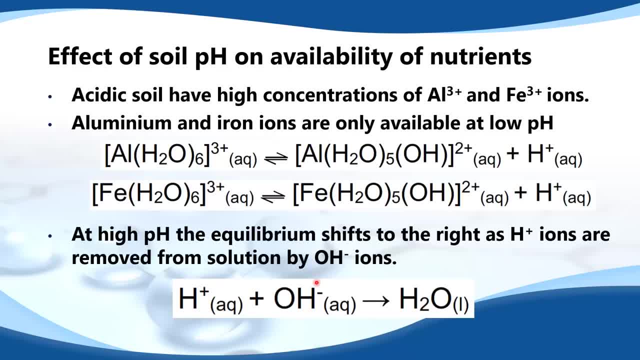 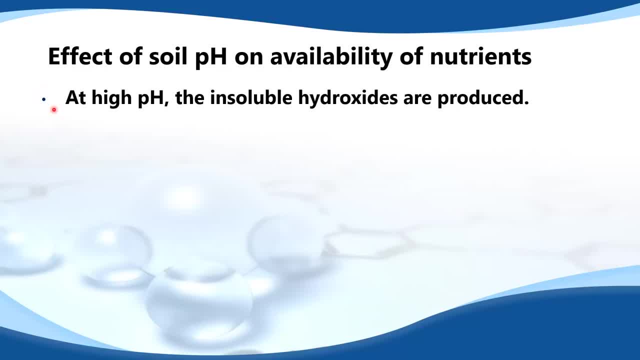 this equation: here H plus ions react with OH negative ions to form a molecule of water At high pH. the insoluble hydroxides are produced. The Al3 plus and Fe3 plus ions are no longer available to plants. So here we have the. 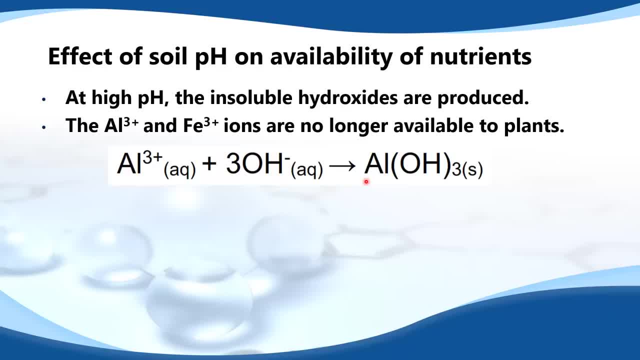 Al3 plus ion reacting with the hydroxide ion to form the insoluble aluminium hydroxide. And here's the Fe3 plus reacting with OH negative to form the insoluble iron hydroxide. And finally the Al3 plus ions at low. 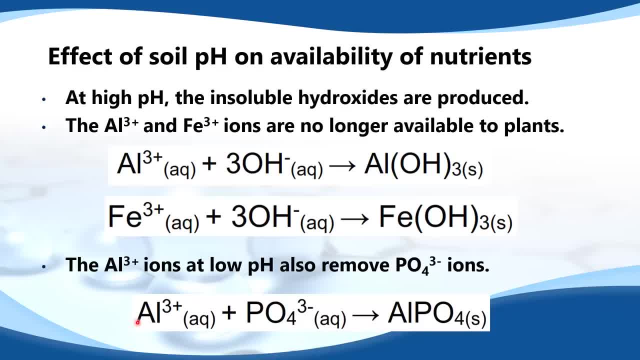 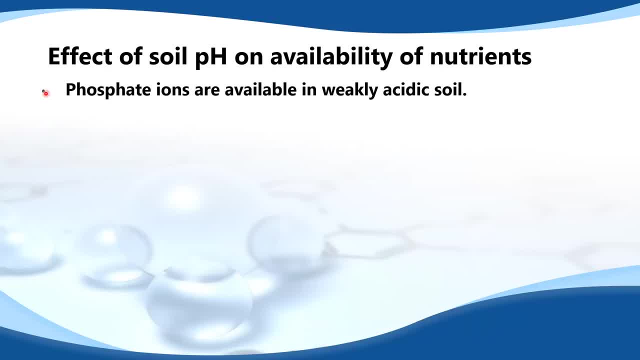 pH also remove phosphate ions. So here we have the aluminium ions reacting with the phosphate ions to form insoluble aluminium phosphate. Next we look at phosphate ions. So phosphate ions are available in weakly acidic soil. Plants absorb inorganic phosphorus as H2PO4 negative, which is present in weakly. 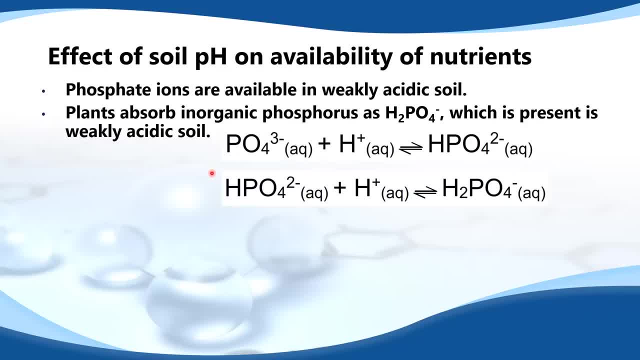 acidic soil. These two equations here show you how the H2PO4 negative is produced and how the H2PO4 negative is produced and how the H2PO4 negative is produced and that then is absorbed by the plants. Phosphate is removed at low pH. 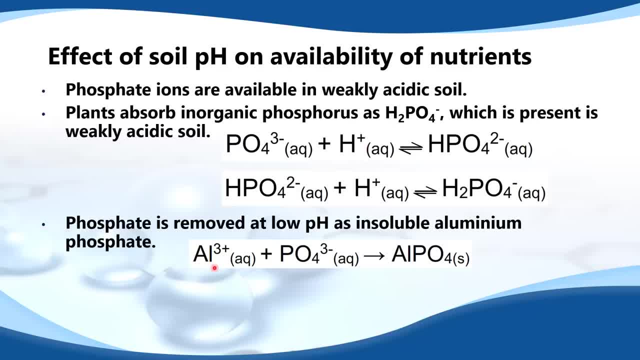 as insoluble aluminium phosphate, And that's the equation that we just looked at. That's Al3 plus plus PO4. 3 negative forms, the insoluble aluminium phosphate. At higher pH, phosphate is removed as insoluble calcium phosphate. So here we. 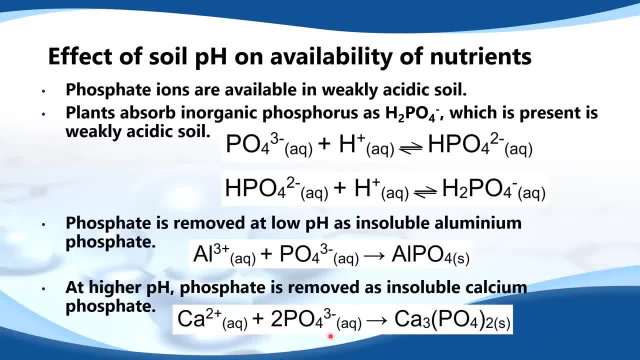 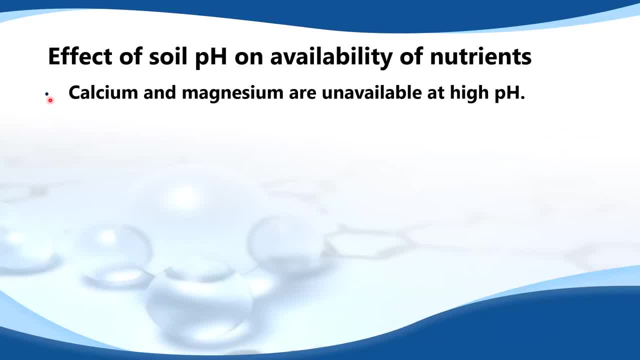 have the Ca2 plus ion reacting with the phosphate ion to form the insoluble calcium phosphate. Next we look at the H2PO4 negative, which is present in the When we look at calcium and magnesium. so calcium and magnesium are unavailable at. 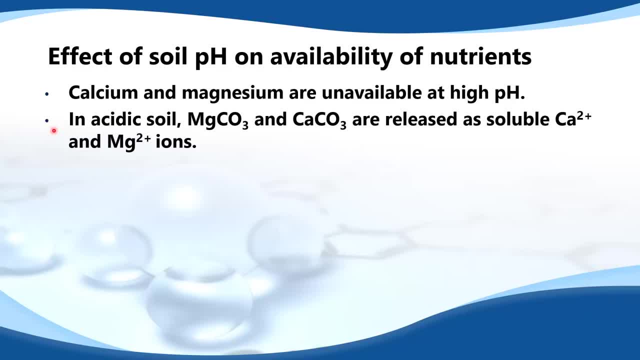 high pH In acidic soil, magnesium carbonate and calcium carbonate are released as soluble Ca2 plus and Mg two plus ions. and here are the two equations. We have calcium carbonate reacting with H plus ion to form those Ca2 plus ions, and here